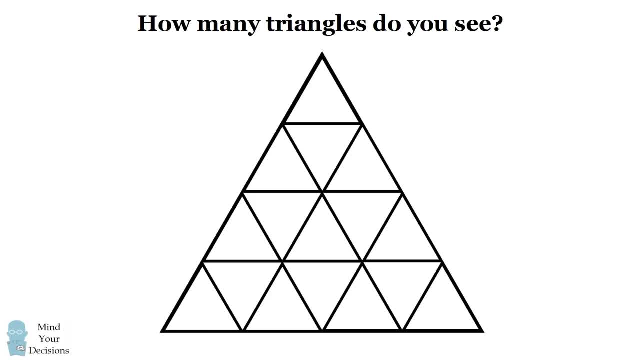 Hi, this is Presh Talwalkar. How many triangles do you see in this picture? Give this problem a try and, when you're ready, keep watching the video. for the solution, We need to count the number of triangles very carefully. We'll first consider triangles which. 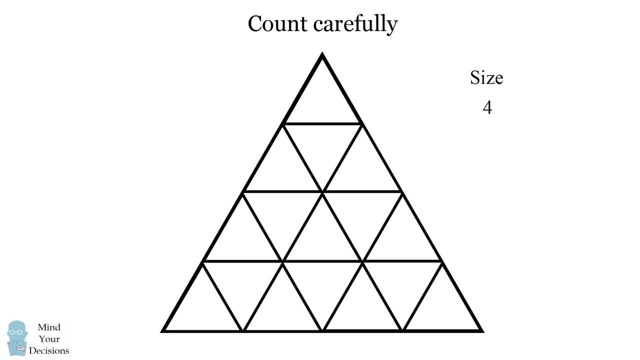 have a size of four, which means its side length is equal to four times the smallest triangle. There's exactly one triangle of this type and this triangle is facing upward. Let's continue counting only the number of triangles which are facing upward. Let's count the number of triangles. 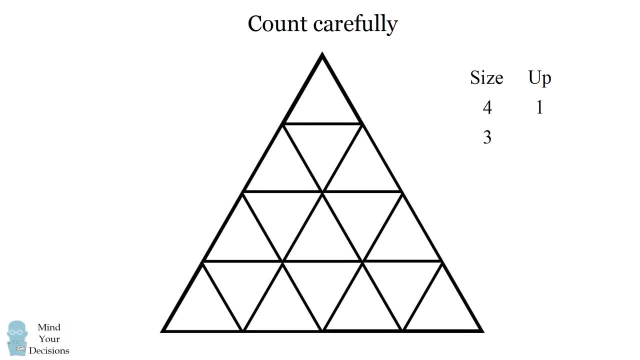 which have size three. In the bottom row there are two of these triangles and one row above that there's one. So that makes for a total of three triangles of size three facing up. How many triangles are there of size two facing up? The bottom row has three. the next row has two. 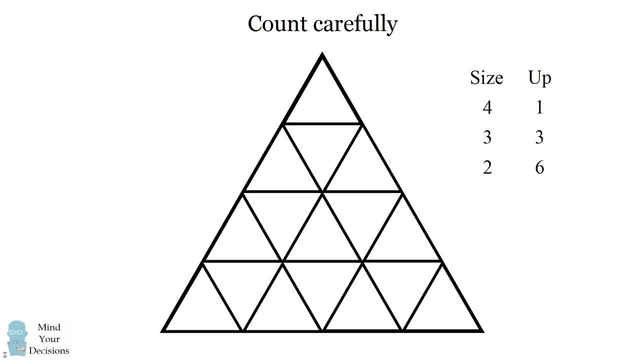 and one row above that has one. Three triangles are facing up. Three plus two plus one is six. Finally, we count the number of triangles of size one facing up. The bottom row has four, the next row has three, the next row has two and the top row 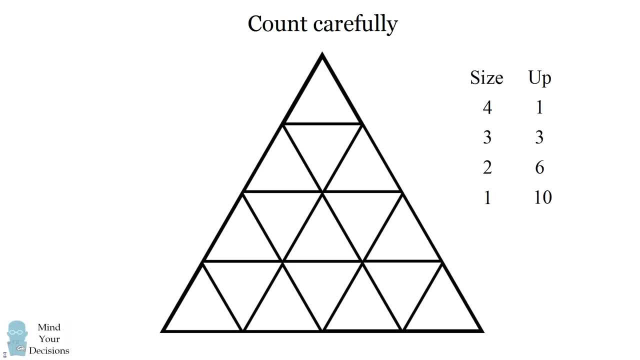 has one. Four plus three plus two plus one is equal to ten. Now we need to count the number of triangles which are facing down. We'll start by counting the number of triangles of size one. The bottom row has three, the next row has two and the row above that has one. 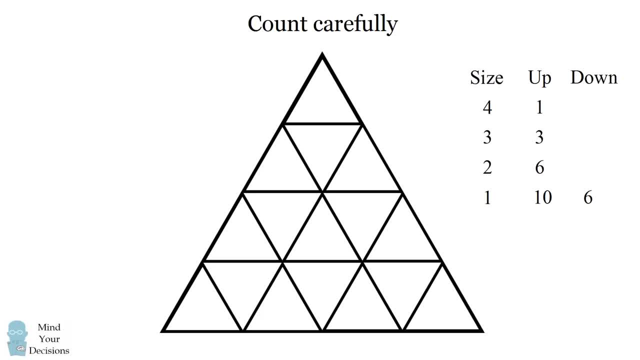 Three plus two plus one is equal to six. Now we count the number of triangles of size two facing down, and there's exactly one. Now, as you can see, this is the largest sized triangle that's facing down. so there are no triangles of size three or four facing down. 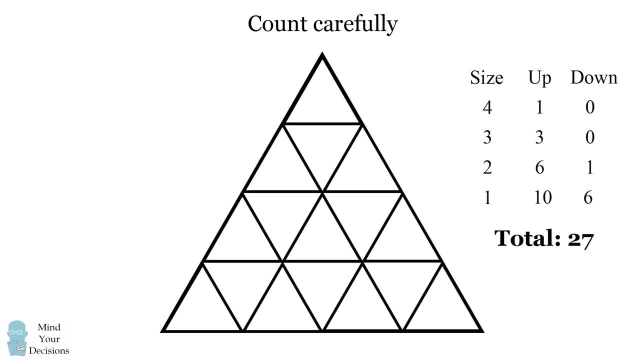 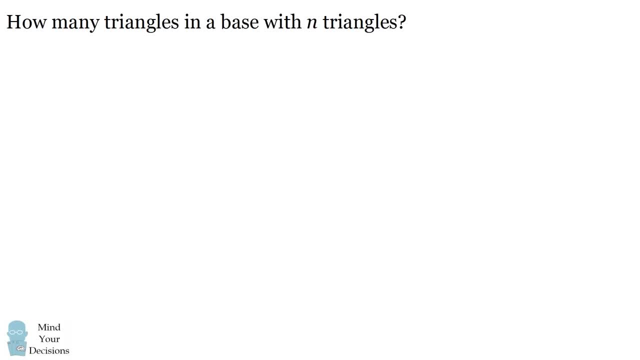 So we've now listed out all the triangles and we can total this up To get that there are twenty-seven triangles in this picture. Now what would happen if we want to generalize this for a base that has n smaller triangles? Well, we found a pattern in the shape we just saw. 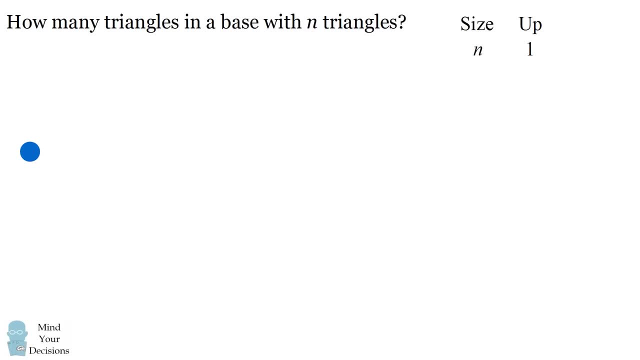 The number of triangles facing up of size n. the largest size was equal to one. The next size: there were two, more of them. The next size: there were more of them, according to this shape. Each time we were adding the next number in the sequence. 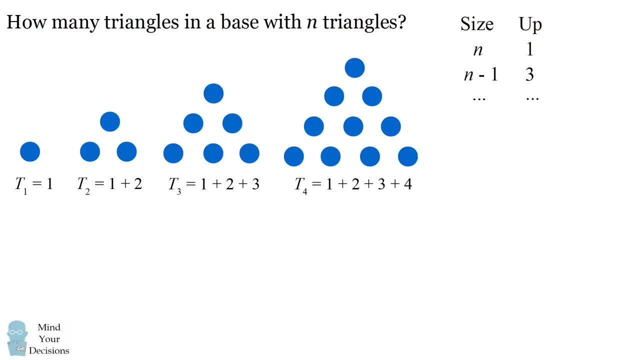 These are the triangular numbers, which are the shapes you can form that have a triangular arrangement of shapes, and they're equal to the sum of the numbers from one to n. The triangles of the smallest size, one, were equal to the triangular number of size n. 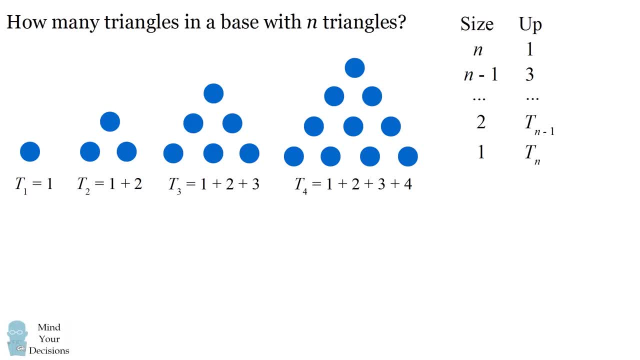 Now in many videos we've figured out the way to sum up the numbers from one to n, and this is the triangular formula number, which is equal to n times n plus one over two. To count the number of triangles facing down, we start from the triangles of size one. 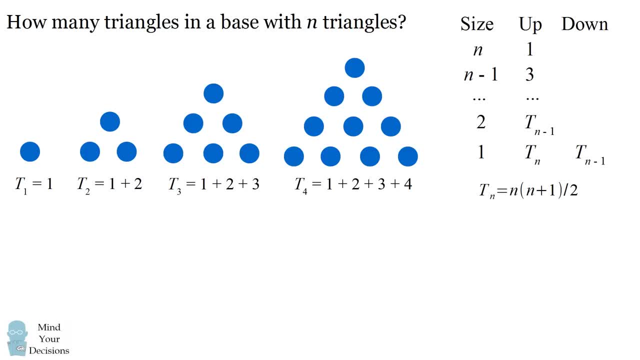 This will be offset by one. So we start out with triangular number of n minus one. To get to the next size of two, we have to offset it by two, because each time the row is decreasing in size. So this is going to go about half way up and then the largest two sizes, many of the 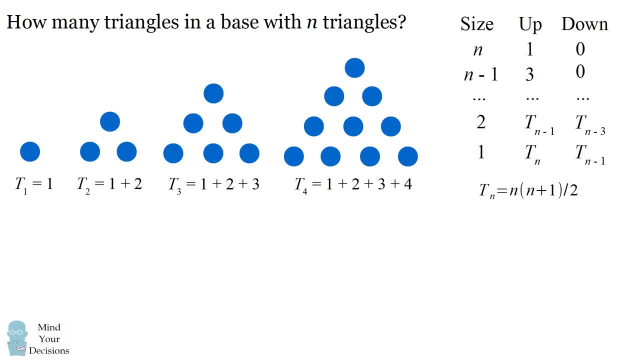 largest sizes. we're going to have zero triangles facing down. So this is going to go about half way up, and then the largest two sizes, many of the largest two sizes. we're going to have zero triangles facing down. So now we've figured out a pattern in how to count the number of triangles of each size. 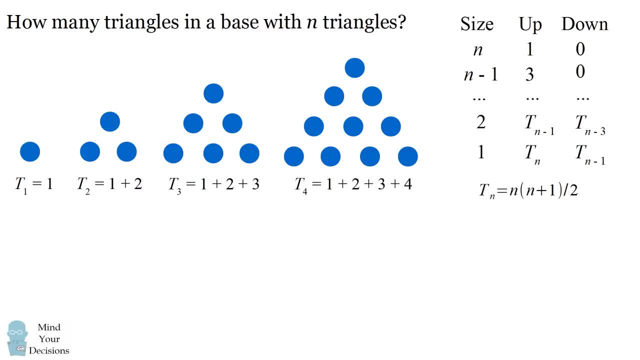 and we have a formula for the number of triangular numbers equal to n times n plus one over two. So this is actually going to vary whether you have n equal, n is going to be even or n is going to be odd. but there's a nice way you can summarize this. if you add up all these, 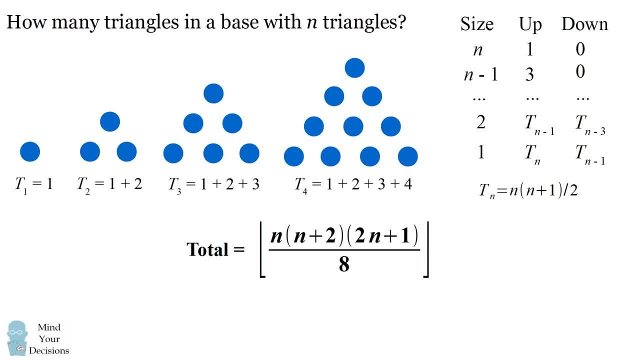 numbers. The total number of triangles is going to be n times n plus two times two, n plus one, all over eight rounded down. So this is going to be n times n plus two times two, n plus one, all over eight rounded down. 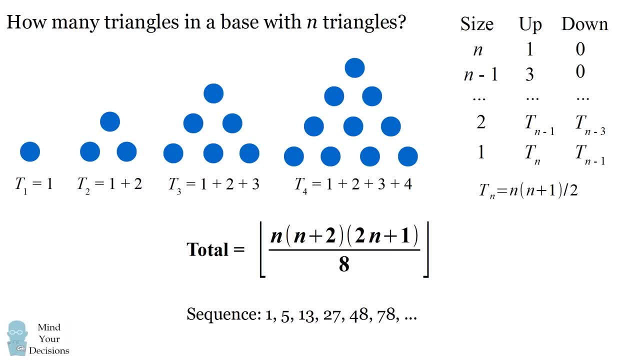 This will give you the number of triangles. it's actually a sequence: The number of triangles formed. if you have this equilateral grid of triangles, the sequence starts out: one, five, thirteen, twenty-seven was what we had when we had four triangles.